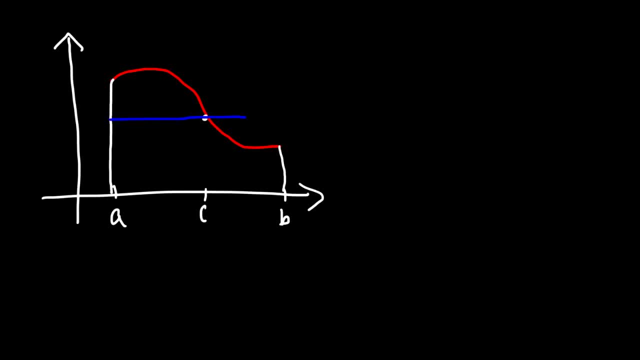 So I'm going to draw the rectangle in blue. So the area of that rectangle is equal to the area under the curve from a to b. And so if the function is continuous on the closed interval a, b and if c is in that interval, then according to the mean value theorem, the definite integral of f of x- dx from a to b is equal to f of c times a to b. 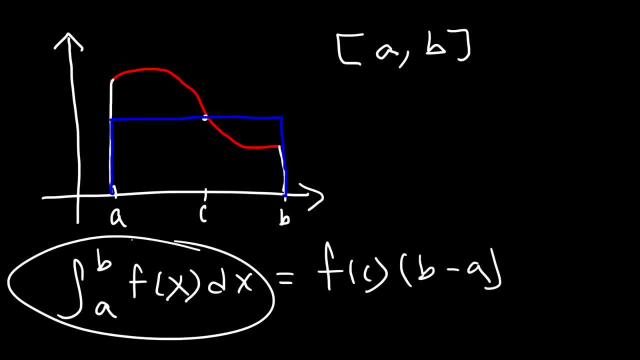 So b minus a. So the definite integral represents the area under the curve in red. So that's the definite integral, So it's the area of the curve And f of c times b minus a. b minus a represents the width of the rectangle And f of c, that's a y value that represents basically the height of the rectangle. 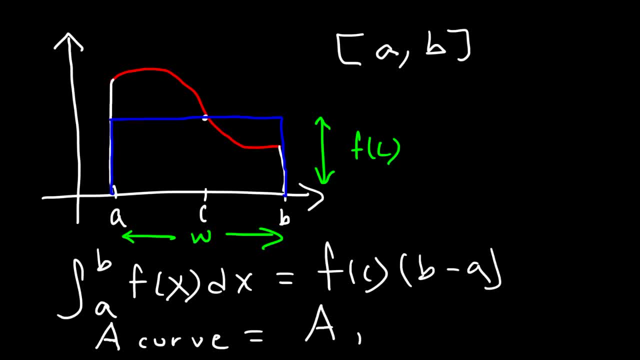 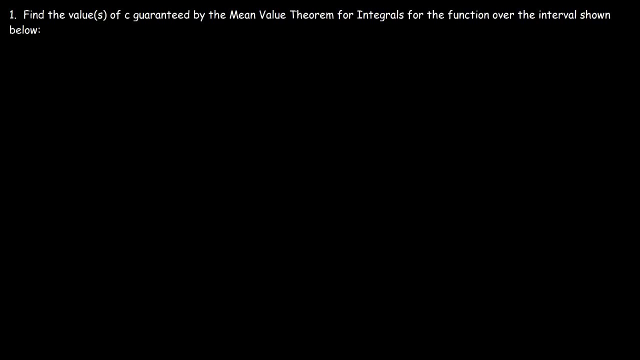 Width times height. that gives us the area of the rectangle. So according to the mean value theorem, at some point c, the area of the rectangle is equal to the area under the curve And f of c represents the average value. Now let's say that f of x is equal to x squared over the interval 0 to 4.. 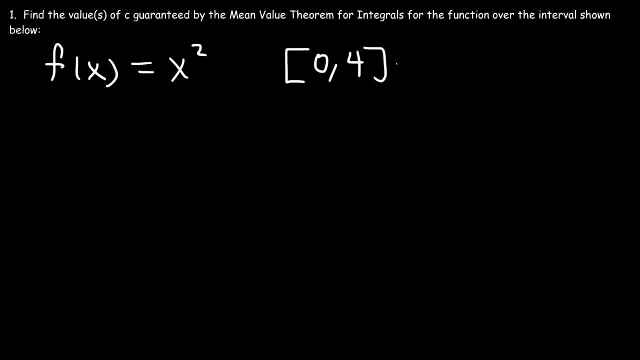 Find the value of c guaranteed by the matrix. This is the mean value theorem for integrals in this function. So let's start with a formula. So the area under the curve is equal to the area of the rectangle. So f of c times b minus a. 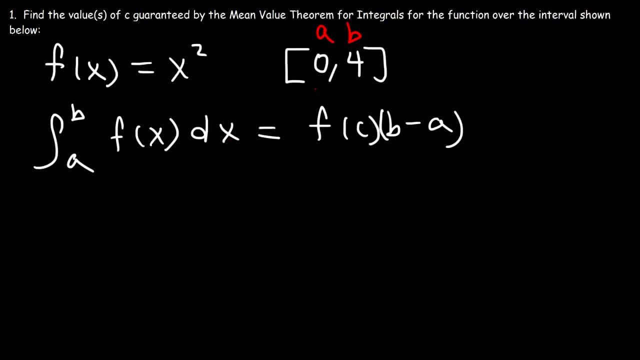 Now a in this example is 0 and b is 4.. So this is going to be the integral from 0 to 4.. And f of x is x squared over the interval 0 to 4.. So f of x is x squared. 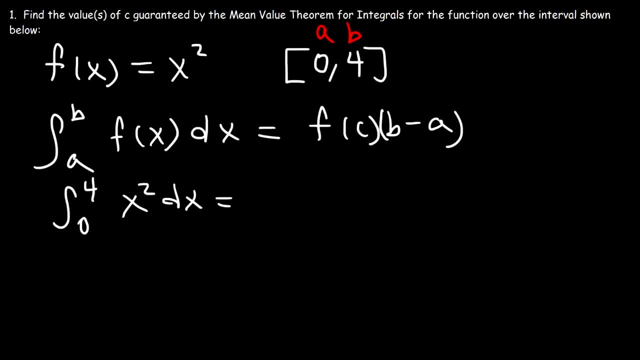 f of c. well, if f of x is x squared, what is f of c? So if you plug in c into that equation, f of c is going to be c squared, And then we have b minus a, So that's going to be 4 minus 0.. 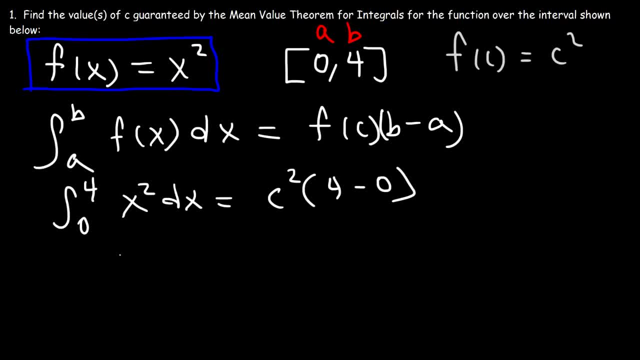 Now, on the left, let's find the antiderivative of x squared. So, using the power rule, it's going to be x cubed over 3, evaluated from 4 to 0.. On the right, we simply have 4c squared. 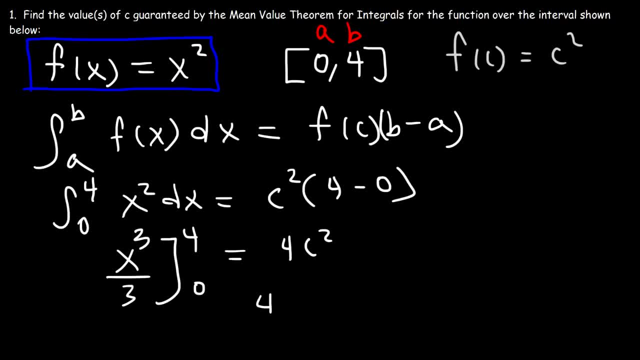 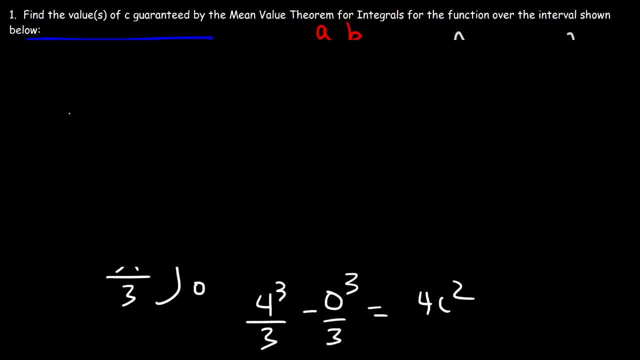 Now let's focus on the left side. If we plug in 4, it's going to be 4 to the 3rd over 3.. And then if we plug in 0, that's just going to be 0. Now 4 to the 3rd is 64.. 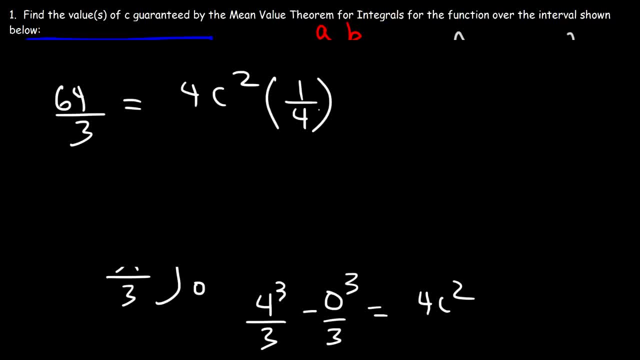 And so we have this. Let's multiply both sides by 1.. 64 divided by 4 is 16.. So 16 over 3 is equal to c squared. Now let's take the square root of both sides. The square root of 16 is 4.. 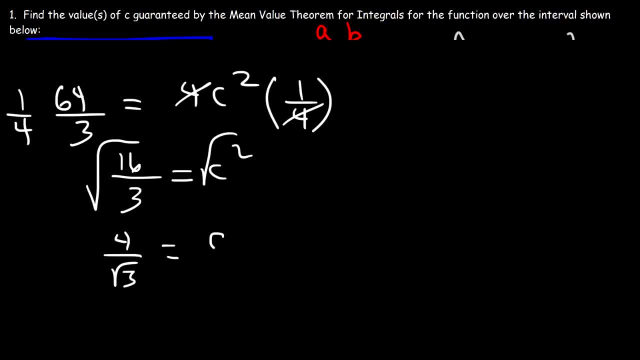 So we have 4 over square root 3. And that's equal to c. But this is going to be plus or minus. Now let's rationalize that value. The final answer is going to be plus or minus 4, square root 3 over 3.. 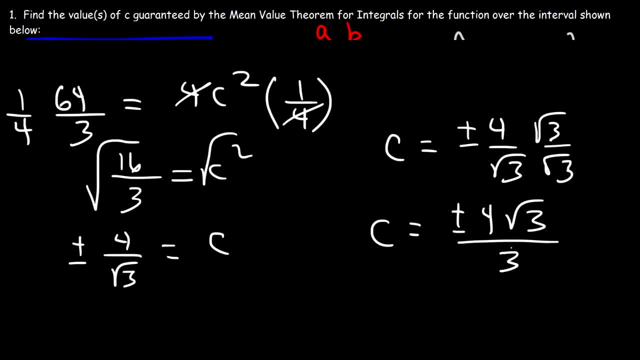 Now to get a decimal value of that. this is plus or minus 2.309.. Now c has to be in the interval a to b, 0 to 4. Positive 2.309 is in that interval, but not negative 2.309.. 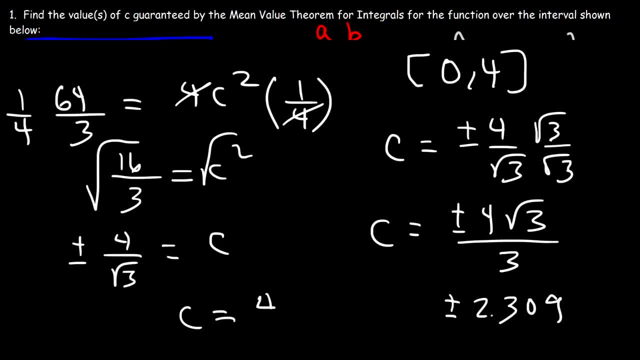 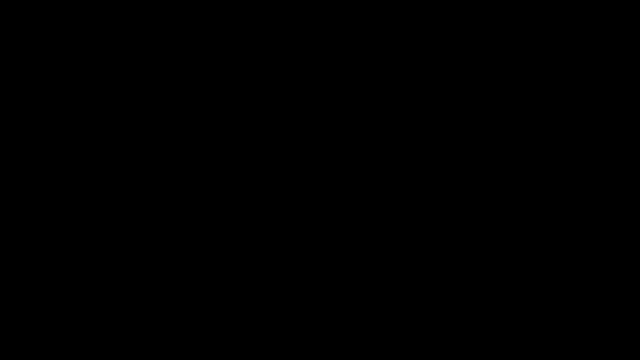 So the c that we're looking for is positive: 4 square root 3 over 3.. And so this is the answer. Let's try another problem. Let's say that f of x is equal to the square root of x on the interval from 1 to 9.. 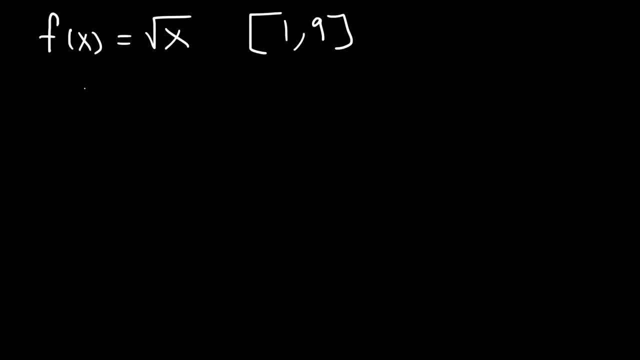 Go ahead and calculate the value of c for this problem. So let's start with the formula. In this example, a is 1, b is 9.. So we have the definite integral from 1 to 9.. f of x is the square root of x. 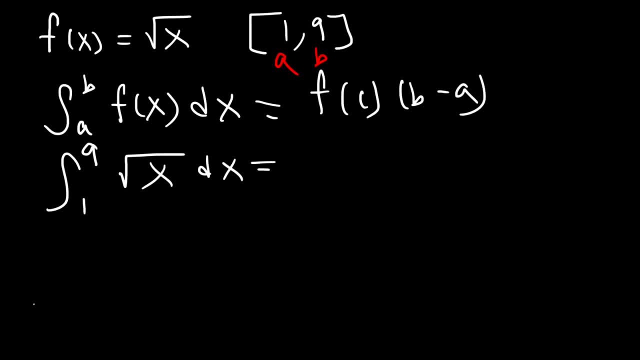 And f of c. all you got to do is replace x with c, So that's going to be the square root of c, And then b minus a, 9 minus 1.. Now let's replace the square root of x with c. 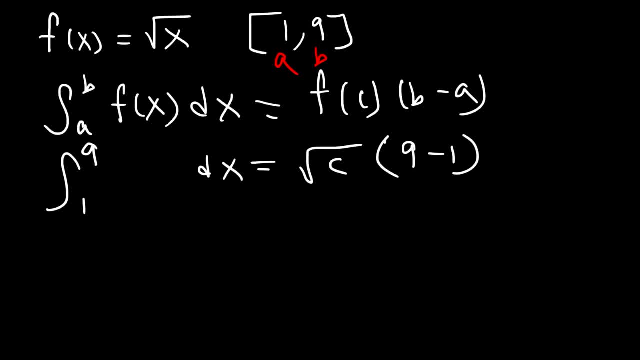 Now let's replace the square root of x with x to the 1 half, Because we need to rewrite it in order to integrate it. So, using the power rule, 1 half plus 1 is 3 over 2. And instead of dividing it by 3 over 2, it's the same as multiplying it by 2 over 3.. 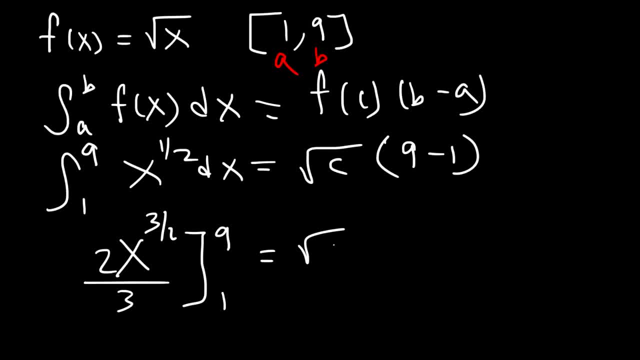 Let's evaluate it from 1 to 9.. And then 9 minus 1 is 8.. So on the left we have 2 times 3.. So 9 times 9 raised to the 3 over 2 over 3 minus 2 times 1 raised to the 3 over 2 over 3.. 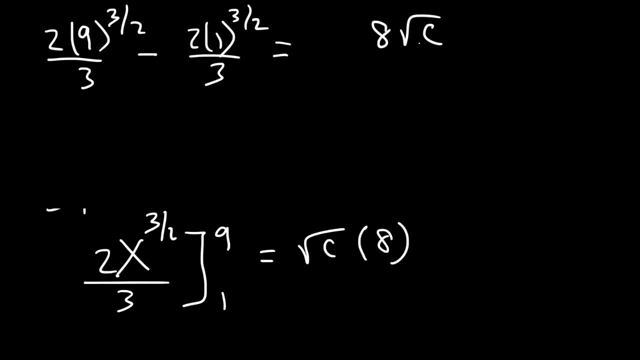 And that's equal to 8 square root c. Now what is 9 raised to the 3 over 2?? How can we evaluate that fractional exponent? So anytime you have rational exponents, it's helpful if you split it. 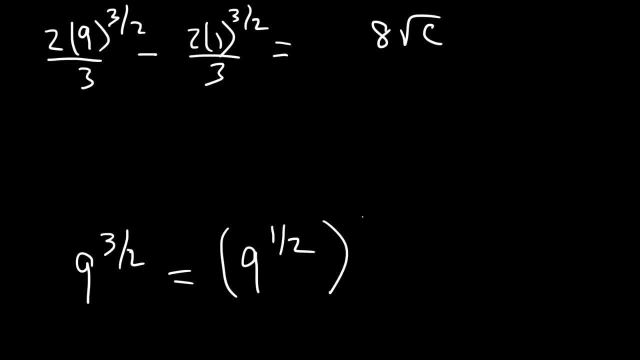 This is the same as 9 raised to the 1 half Raised to the 3.. When you raise one exponent to another, you need to multiply them A half times. 3 is 3 halves, So 9 to the 1 half is basically the same as the square root of 9, which is 3.. 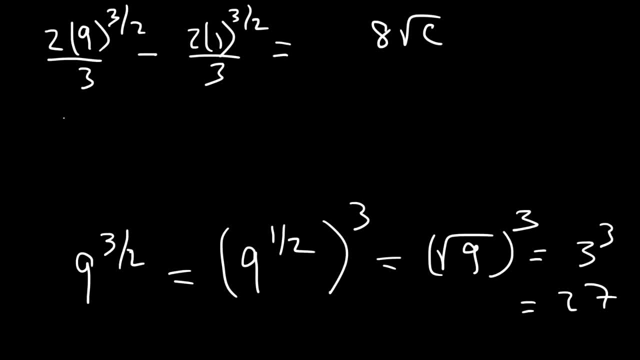 And 3 to the 3rd is 27.. So therefore, we have 2 thirds of 27 and then minus 2 thirds of 1.. We can factor out 2 thirds and make it easier, Or we could just multiply 2 and 27.. 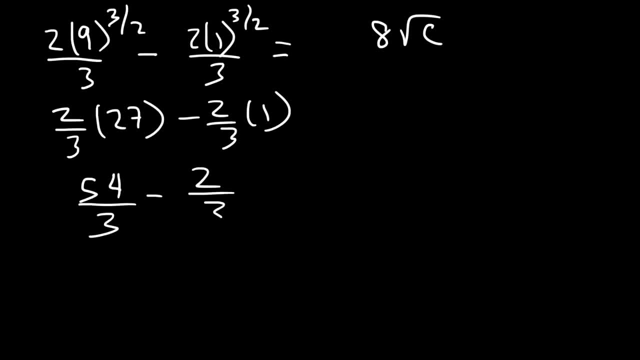 2 times 27 is 54. And then minus 2 over 3.. 54 minus 2 is 52. And so, right now, this is what we have. Now what we need to do is divide both sides by 8, or multiply both sides by 1 over 8.. 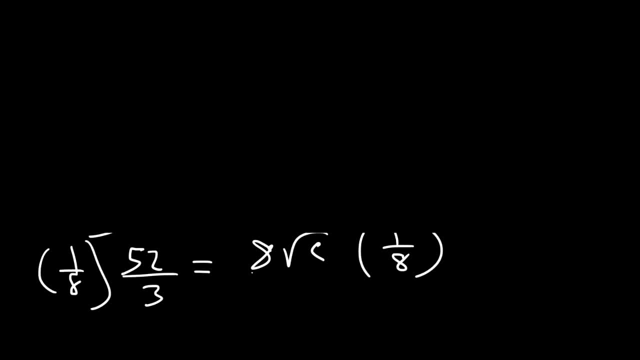 So we could cancel these 8s. On the right, we could break down 52 into 13 times 4. And 8 is 4 times 2. And let's not forget the 3. So we could cancel a 4.. 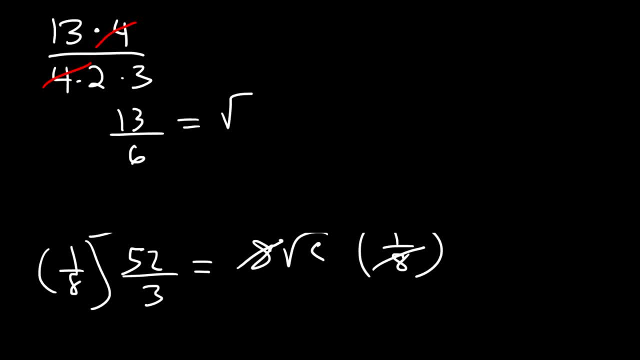 And so we have: 13 over 6 is equal to the square root of C. So now we need to take the square of both sides: 13 squared is 169.. 6 squared is 36. And that's equal to C. 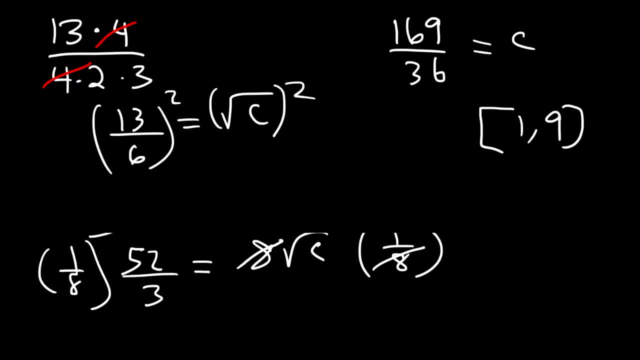 Now we need to make sure that it's in the interval A to B And this problem 1 to 9.. So let's get the decimal value of 169 over 36.. So as a decimal that's about 4.694.. 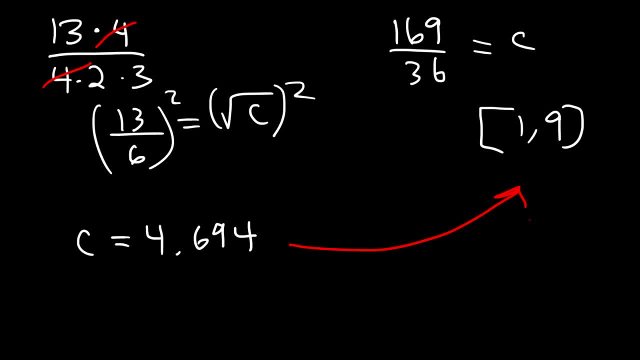 So that's definitely in this interval. So this is, That's the answer. Now let's say that f of x is a linear function And let's say it's 2x plus 3 on the interval from 2 to 10.. 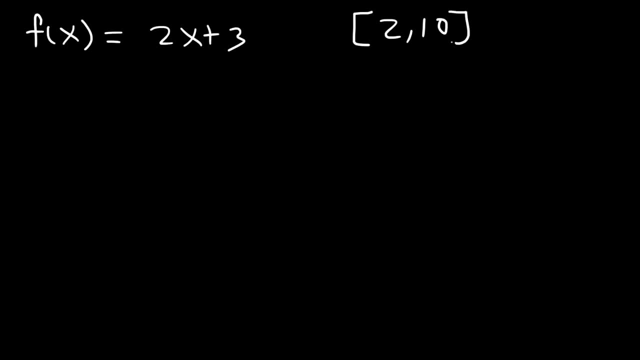 Now, if you had to guess the value of C, what would you say? Now, what is the midpoint of 2 and 10?? To find the midpoint, we can average the two values: 2 plus 10 is 12.. 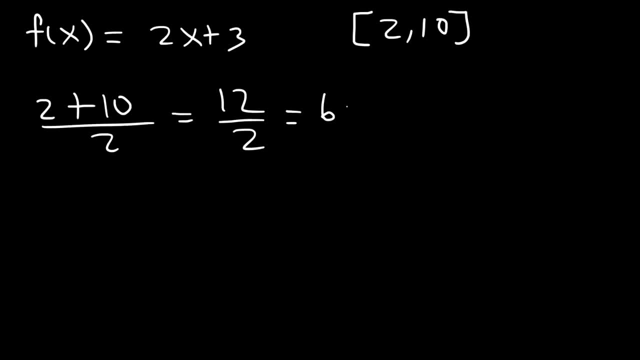 And 12 divided by 2 is 6.. Do you think C will be less than 6, equal to 6, or greater than 6?? Now for linear functions. the C value will be equal to the midpoint value. Now let's confirm it. 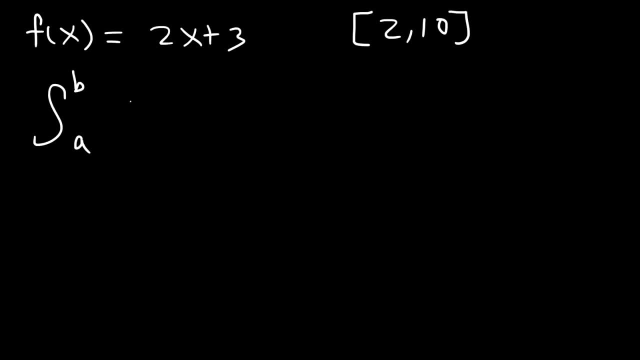 So let's start with our original formula And then let's plug in. Let's plug in What we have. So A is 2.. B is 10.. F of x is 2x plus 3. And so f of C is going to be 2C plus 3.. 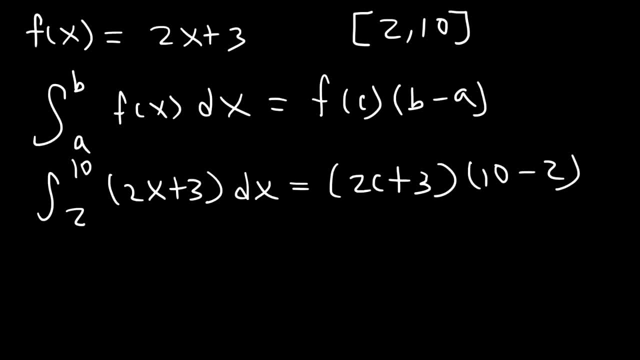 And then B minus A, That's 10 minus 2.. Now the antiderivative of x is x squared over 2.. And for 3, it's 3x. Evaluate it from 2 to 10.. Now 2.. 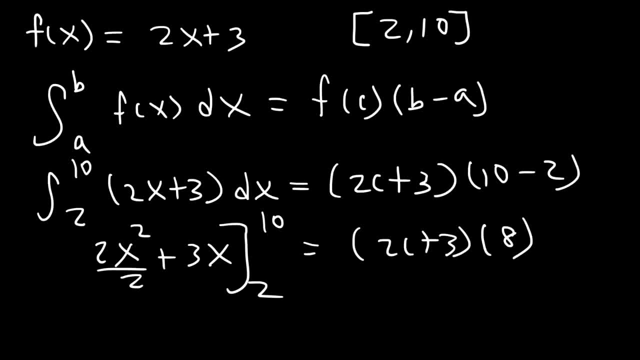 I mean, 10 minus 2 is 8.. So now let's focus. Let's focus on the right side. We could cancel a 2.. And so we have x squared plus 3x. If we plug in 10, that's going to be 10 squared plus 3 times 10.. 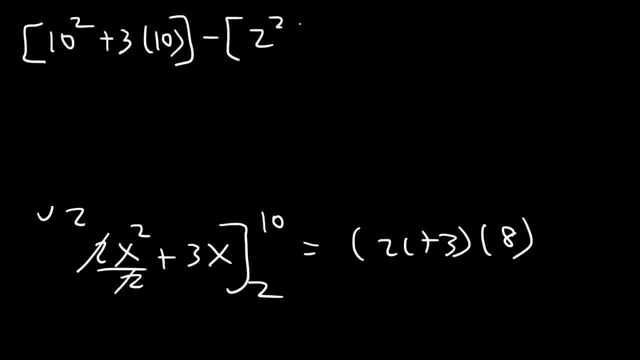 And then minus. we need to plug in 2.. 2 squared plus 3 times 2.. So all of that is equal to 2C plus 3 times 8.. 10 squared is 100.. And 3 times 10 is 30.. 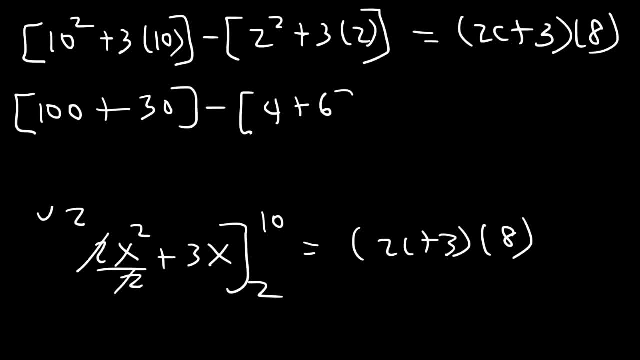 2 squared is 4.. 3 times 2 is 6.. 100 plus 30 is 130.. And 4 plus 6 is 10.. And 130 minus 10 is 120.. So now let's divide both sides by 8.. 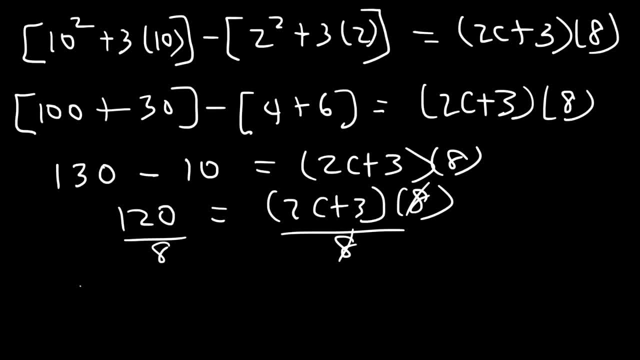 So what's 120 over 8?? Think of 120 as 80 plus 40.. And 80 divided by 8 is 10.. 40 divided by 8 is 5.. So 120 divided by 8 is 15.. 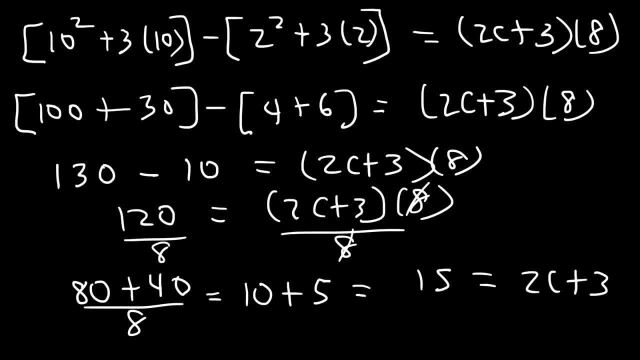 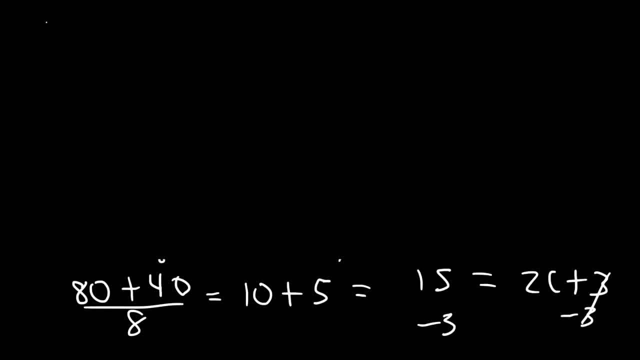 And that's equal to 2C plus 3.. Now let's subtract both sides by 3.. So 50 divided by 8 is 10.. So 15 minus 3 is 12. And that's equal to 2C. 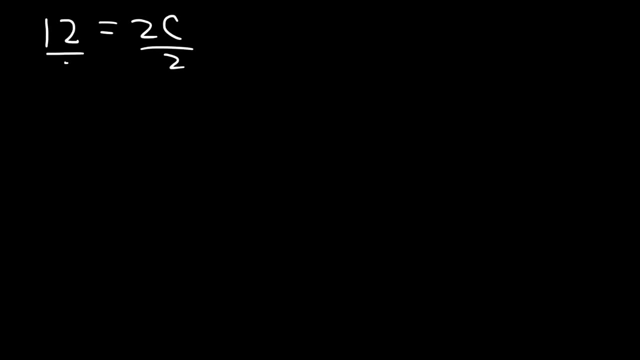 And so if we divide by 2,, we can see that C, in this example, is 6.. And 6 is the midpoint of AB, which is 2 to 10.. And so, for a linear function, the C value, where the area of the rectangle is equal to the area under the curve, is simply the midpoint of AB. 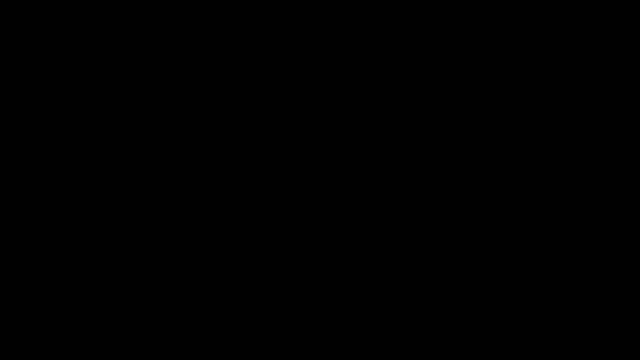 Okay, Now let's compare the three problems that we had. So the first one was X squared, which looked like this. The second one was the square root of X, which looks like that on the right side of the graph. This is just the right half of X squared.